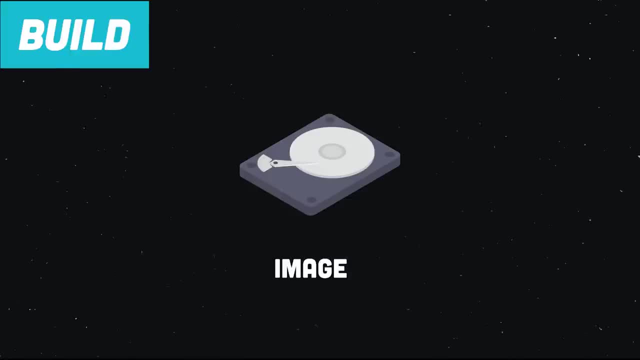 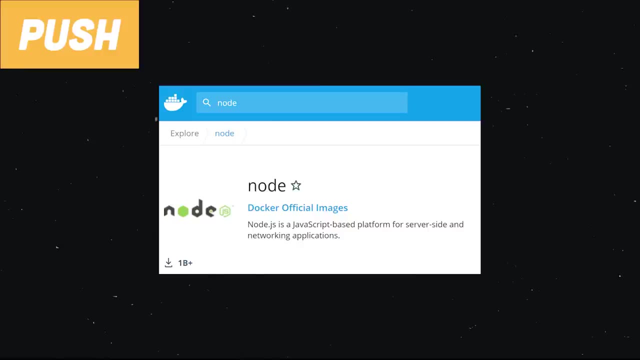 can use the Docker file to rebuild the environment, which is saved as an immutable snapshot known as an image. Images can be uploaded to the cloud in both public and private registries. Then any developer or server that wants to run that software can pull the image down to create. 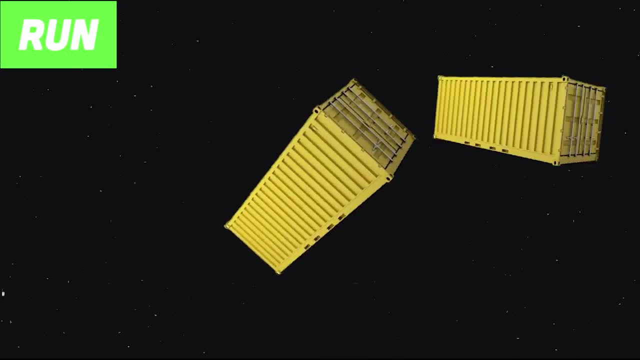 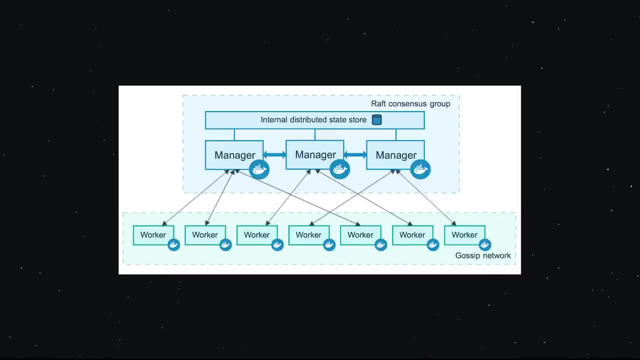 a container which is just a running process of that image. In other words, one image file can be used to spawn the same process multiple times in multiple places, And it's at that point where tools like Kubernetes and Swarm come into play to scale containers to an infinite workload. The best 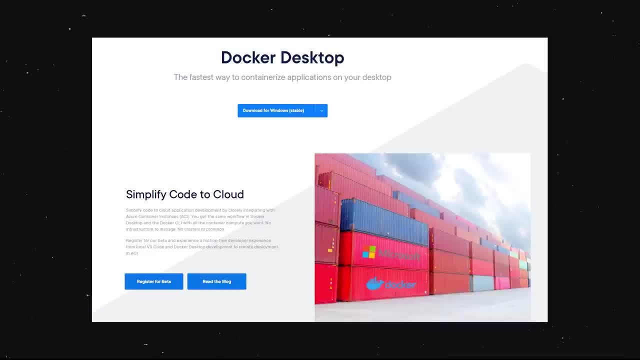 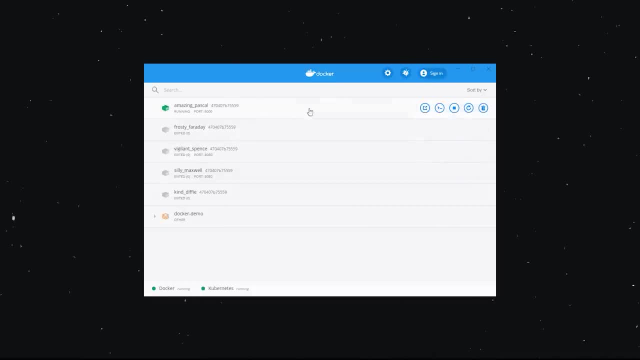 way to really learn Docker is to use it, And to use it we need to install it. If you're on Mac or Windows, I would highly recommend installing the Docker desktop application. It installs everything you need for the command line and also gives you a GUI where you can inspect your running containers. 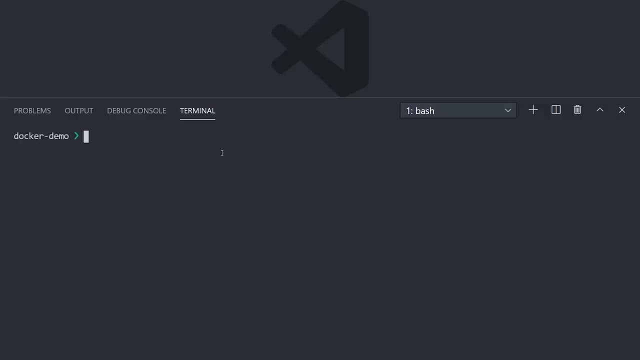 Once installed, you should have access to Docker from the command line, And here's the first command you should memorize: docker ps, which gives you a list of all the running containers on your system. You'll notice how every container has a unique ID and is also linked to an image, And keep in. 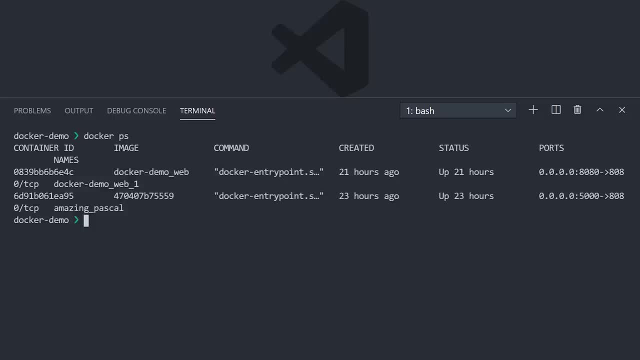 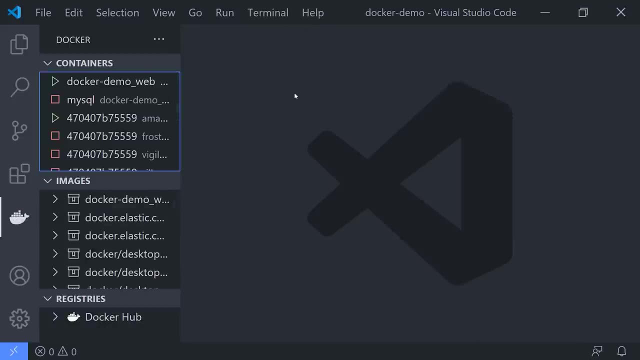 mind, you can find the same information from the GUI as well. Now, the other thing you want to install is the Docker extension for VS code or for your IDE. This will give you language support when you write your Docker files and can also link up to remote registries and a bunch of 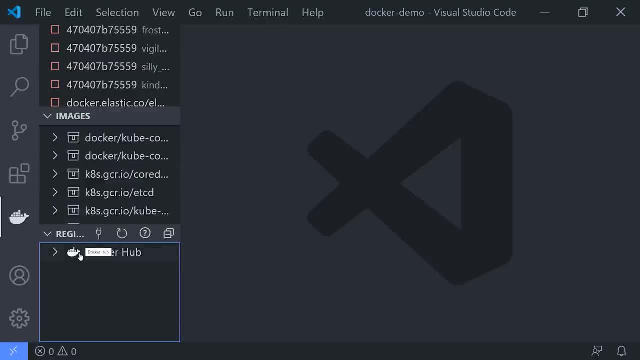 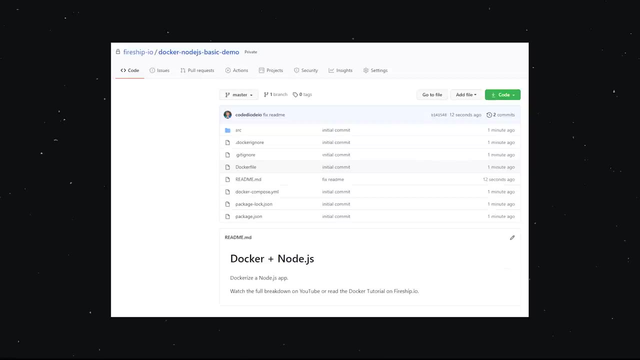 other stuff. Now that we have Docker installed, we can move on to what is probably the most important section of this video, And that's the Docker file, which contains code to build your Docker image and ultimately run your app as a container. Now, to follow along, at this point you can grab my source. 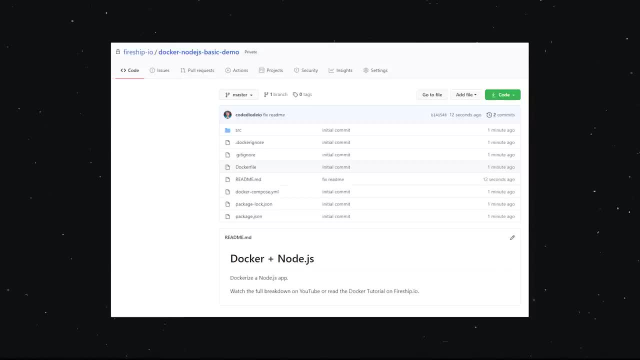 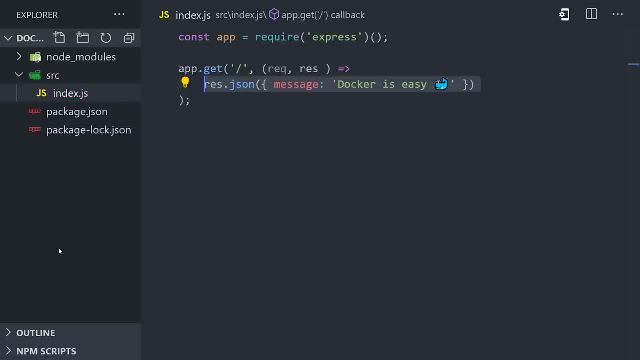 code from GitHub or Fireshipio or, better yet, use your own application as a starting point. In this case, I just have a single indexjs file that exposes an API endpoint that sends back a response. Docker is easy. Then we expose our app using the port environment variable, and that'll come into play later. 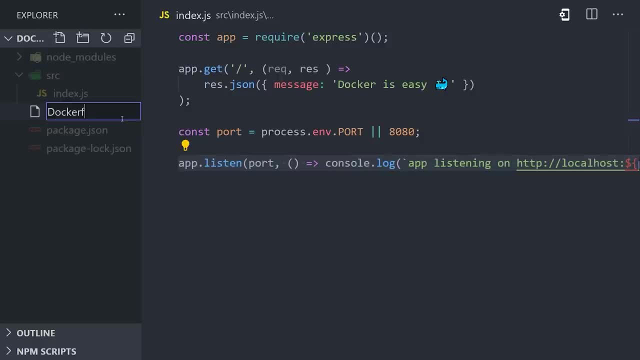 The question we're faced with now is: how do we Dockerize this app? We'll start by creating a Docker file in the root of the project. The first instruction in our Docker file is from, and if you hover over it, it will give you some documentation about what it does. 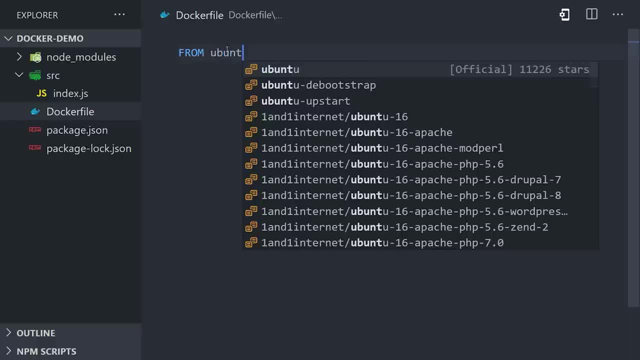 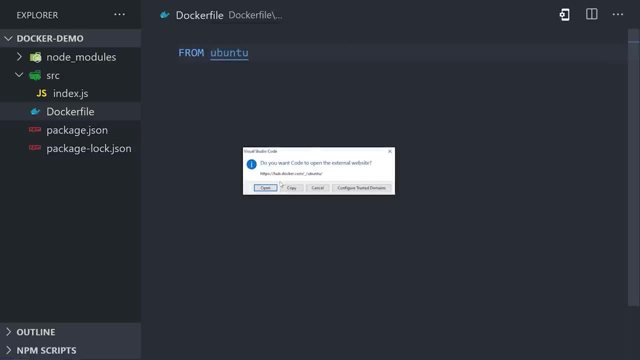 You could start from scratch with nothing but the Docker runtime. However, most Docker files will start with a specific base image. For example, when I type Ubuntu, you'll notice it's underlined, And when I control, click it, it will take me to all the base images for this. 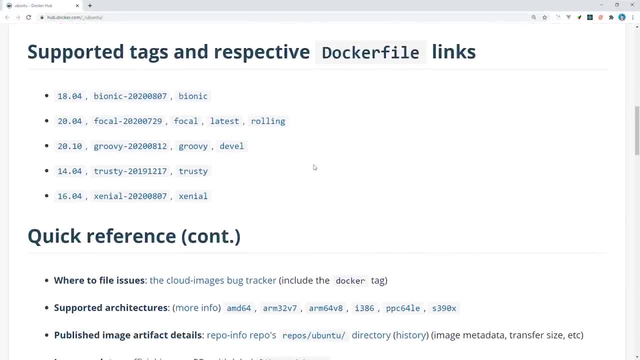 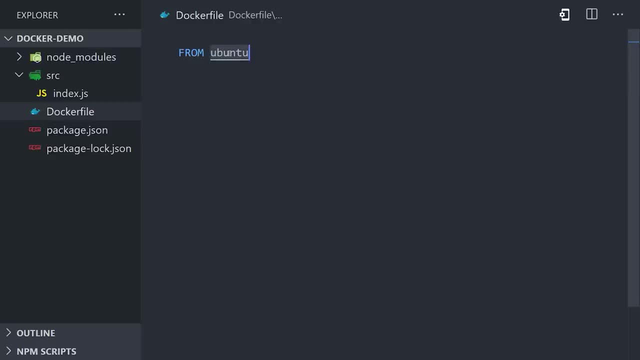 and then you'll notice it supports a variety of different tags, which are just different variations on this base image. Ubuntu doesn't have Nodejs installed by default. We could still use this image and install Nodejs manually. However, there is a better option and that's to use the 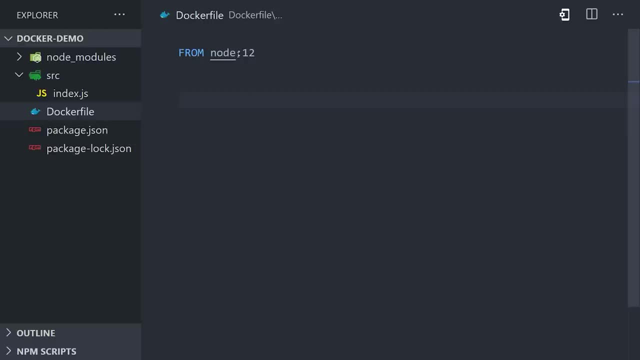 officially supported Nodejs image. We'll go ahead and use the Node version 12 base image, which will give us everything we need to start working with Node in this environment. The next thing we'll want to do is add our app source code to the image- The working directory. 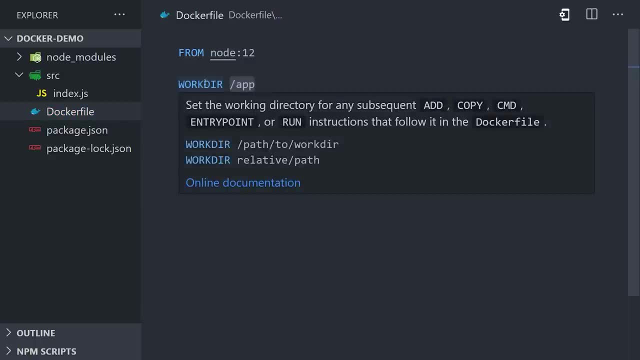 instruction is kind of like when you CD into a directory. Now, any subsequent instructions in our Docker file will start from this app directory. Now, at this point there is something very important that you need to understand, and that's that every instruction in this Docker file is: 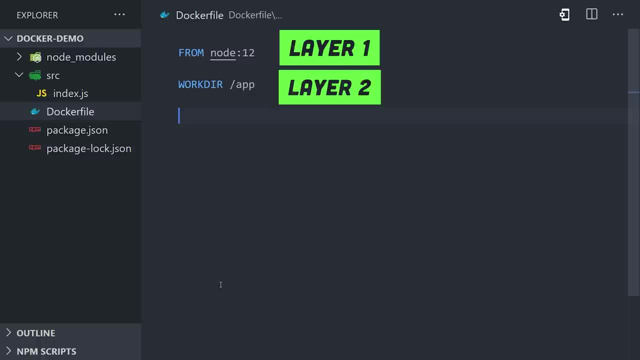 considered its own step or layer. In order to keep things efficient, Docker will attempt to cache layers if nothing is actually changed. Now, normally, when you're working on a Node project, you get your source code and then you install your dependencies, But in Docker, we actually 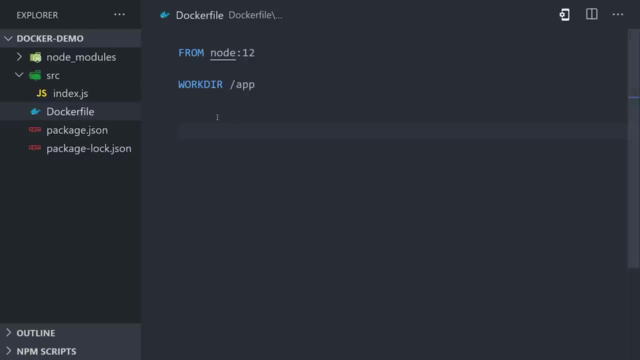 want to install our dependencies first so they can be cached. In other words, we don't want to have to reinstall all of our Node modules every time we change our app source code. In order to do this, we're going to need to install our packagejson, which is our local. 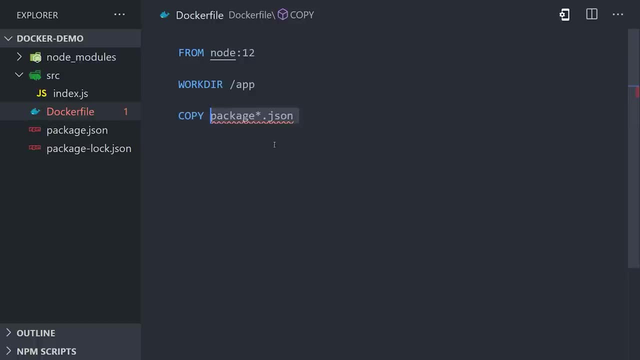 packagejson location. and then the second argument is the place we want to copy it in the container, which is the current working directory, And now that we have a packagejson, we can run the npm install command. This is just like opening a terminal session and running a. 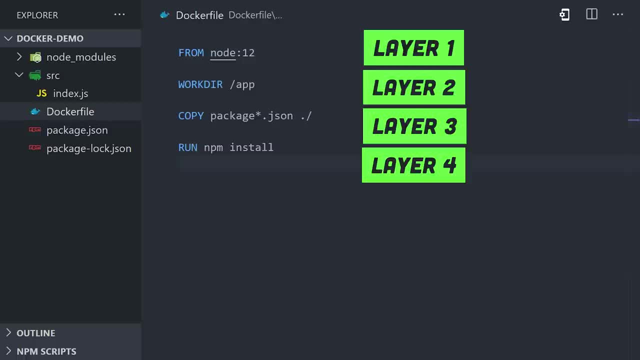 command And when it's finished, the results will be committed to the Docker image as a layer. Now that we have our modules in the image, we can then copy over our source code, which we'll do by copying over all of our local files to the current working directory. 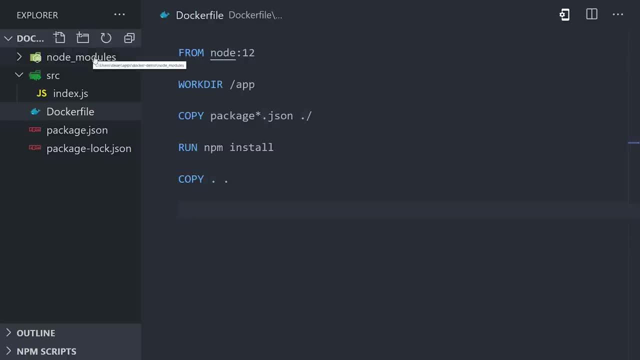 But this actually creates a problem for us, because you'll notice that we have a node modules folder here in our local file system. that would also be copied over to the image and override the node modules that we install there. What we need is some kind of way for Docker. 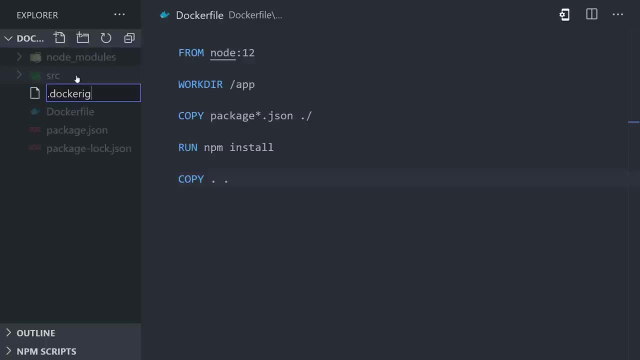 to ignore our local node modules. We can do that by creating a Docker ignore file and adding node modules to it. It works just like a gitignore file, which you've probably seen before. Okay, so at this point we have our source code in the Docker image, but in order to run our code, 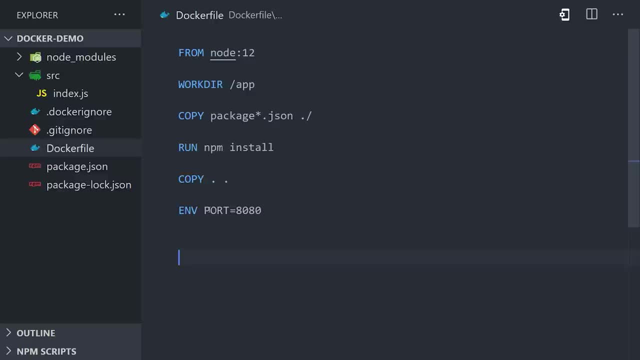 we're using an environment variable. We can set that environment variable in the container using the env instruction. Now, when we actually have a running container, we also want it to be listening on port 8080, so we can access the Nodejs express app publicly And we'll look. 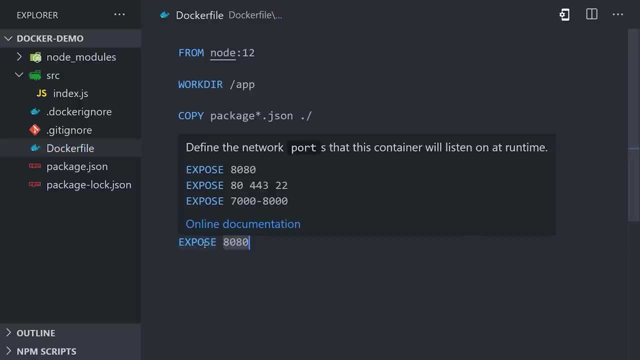 at port. some more detail in just a minute- when we run the container- And that brings us to our final instruction command- There can only be one of these per Docker file- and it tells the container how to run the actual application, which it does by starting a process to serve. 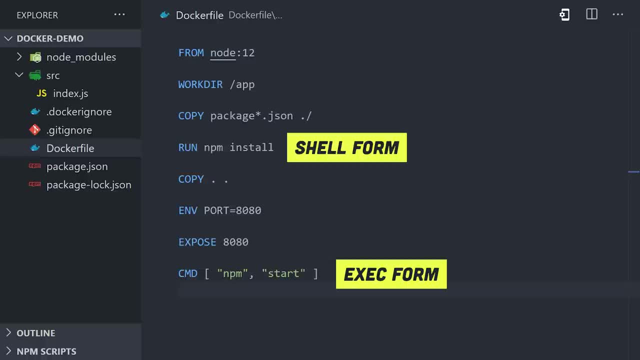 the express app. You'll also notice that, unlike run, we've made this command an array of strings. This is known as exec form, and it's the preferred way to do things. Unlike a command, it doesn't start up a shell session And that's basically all there is to it. We now 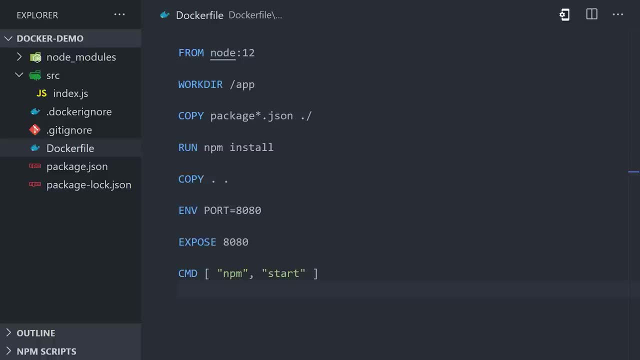 have a full set of instructions for building a Docker image. And that brings us to the next question: How do we build a Docker image? You build a Docker image by running the Docker build command. There's a lot of different options you can pass with the command, but the one you want. 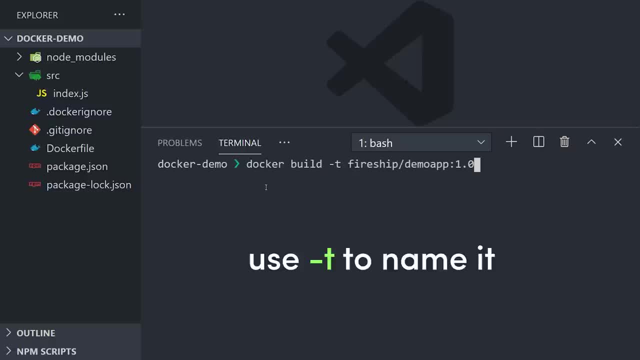 to know for right now is tag or T. This will give your image a name tag that's easy to remember so you can access it later. When defining the tag name, I'd first recommend setting up a username on Docker hub and then do that username, followed by whatever you want to call this image. 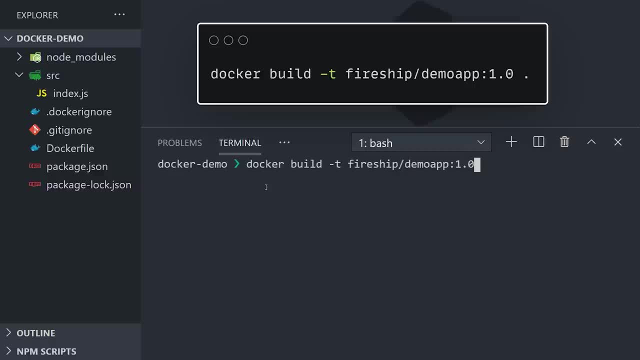 So in my case it would be fire ship slash demo app, And you could also add a version number separated by a colon From there. you simply add the path to your Docker file, which in our case is just a period for the current working directory. When we run it you'll notice it starts with step. 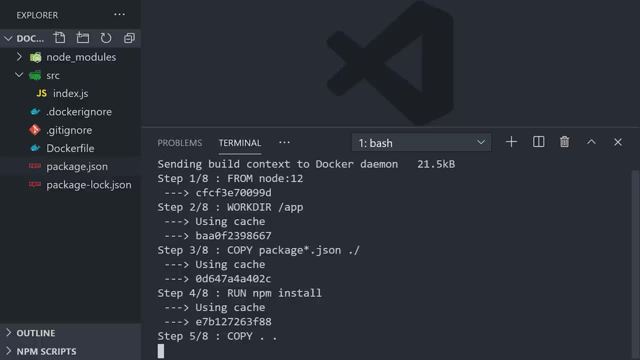 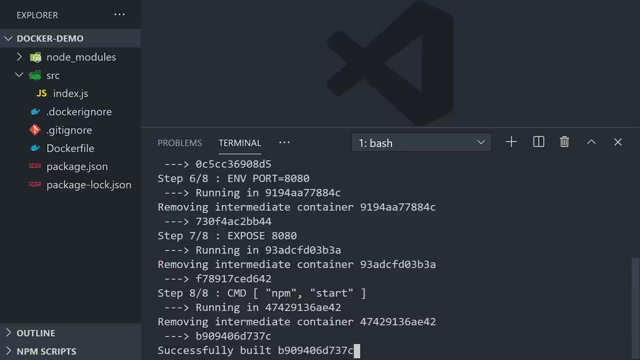 one which is to pull the node 12 image remotely. Then it goes through each step in our Docker file And finally it says successfully built the image ID. And now that we have this image, we can use it as a base image to create other images or we can use it to run containers. 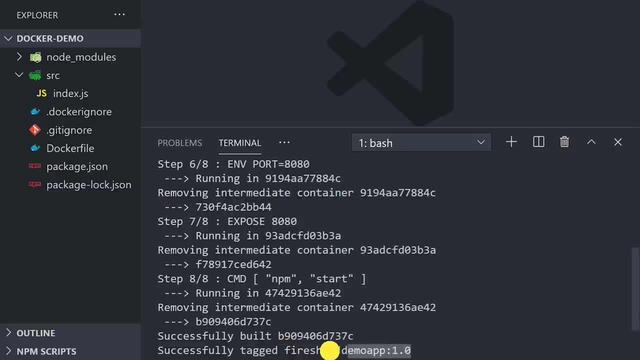 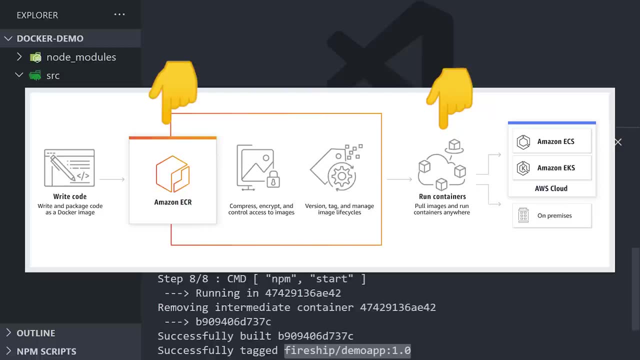 In real life. to use this image, you'll most likely push it to a container registry somewhere that might be Docker hub or your favorite cloud provider, And the command you would use to do that is Docker push in. a developer or server somewhere else in the world could use Docker pull to pull that image back down, But we just want 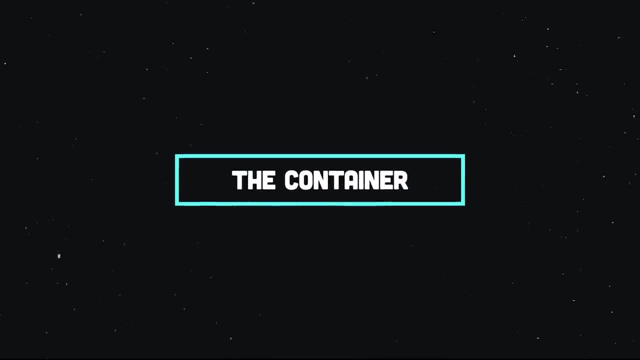 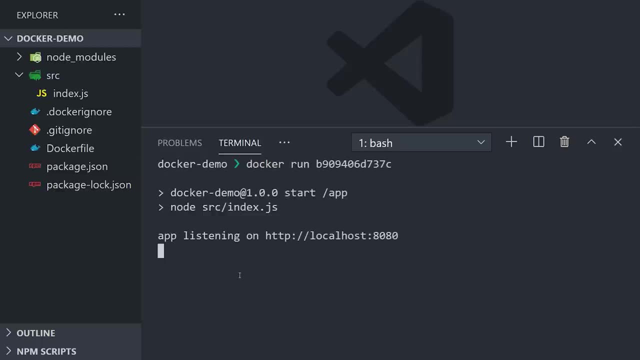 to run it here locally in our system. So let's do that with the Docker run command. we can supply it with the image ID or the tag name And all that does is create a running process called a container And we can see in the terminal it should say: app listening on localhost. 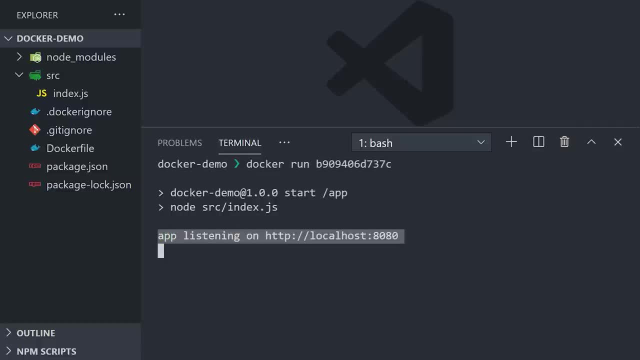 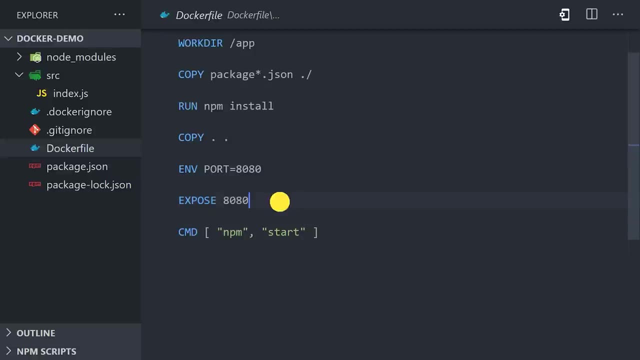 8080. But if we open the browser and go to that address, we don't see anything. So why can't I access my container locally? Remember we exposed port 8080 in our Docker file, but by default it's not accessible to the outside world. Let's refactor our command to use the P. 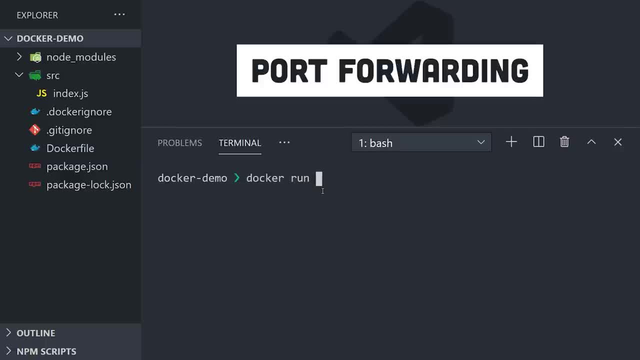 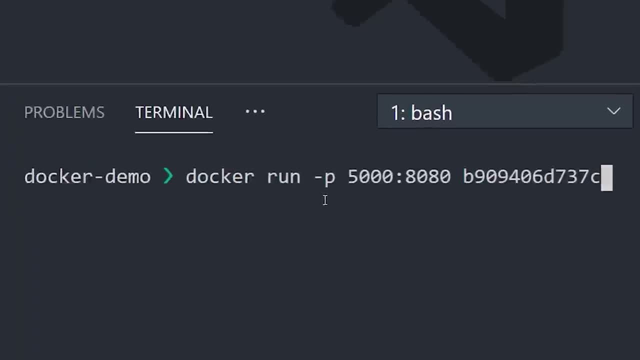 flag to implement port forwarding from the Docker container to our local machine On the left side. we'll map a port on our local machine- 5000. In this case- to a port on the Docker container 8080 on the right side. And now if we open the browser and go to localhost 5000, we'll see the app. 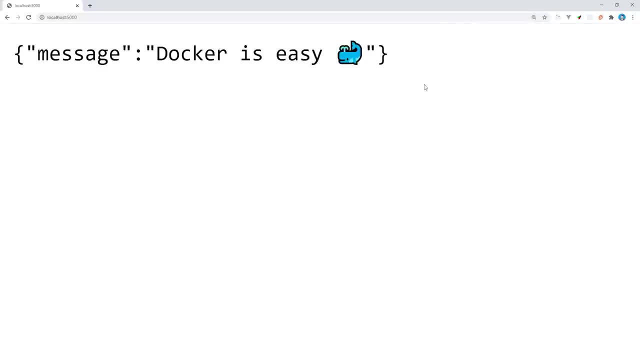 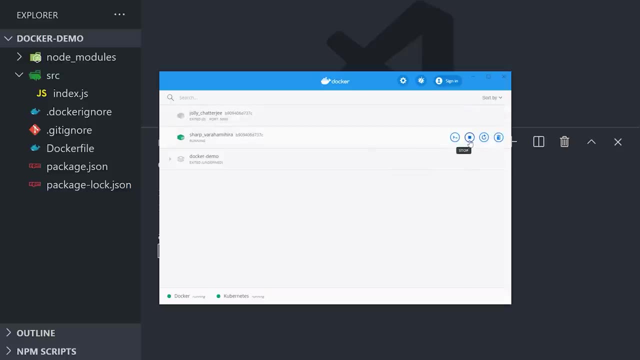 running there. Now, one thing to keep in mind at this point is that the Docker container will still be running even after you close the terminal window. Let's go ahead and open up the dashboard and stop the container. you should actually have two running containers here. if you've been. 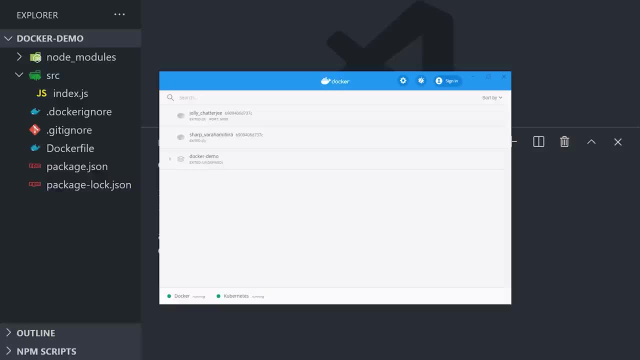 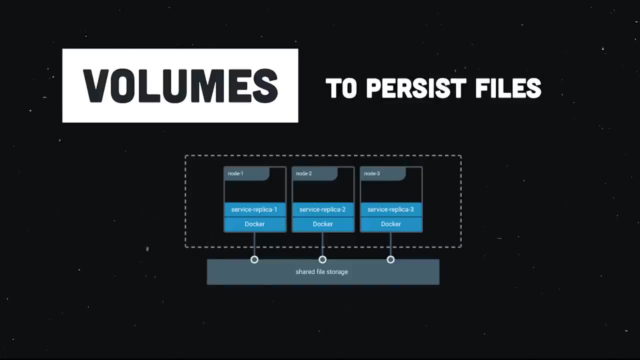 following along. When you stop the container, any state or data that you created inside of it will be lost. But there can be situations where you want to share data across multiple containers, And the preferred way to do that is with volumes. A volume is just a dedicated folder on the host. 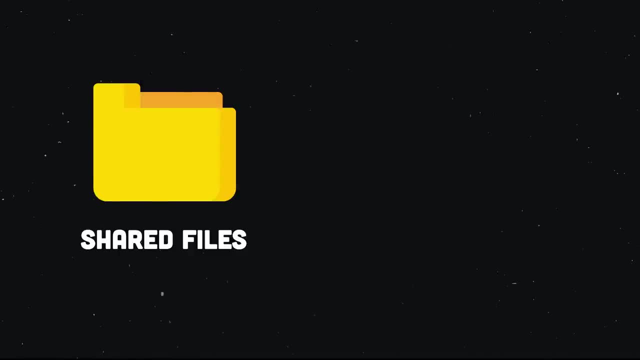 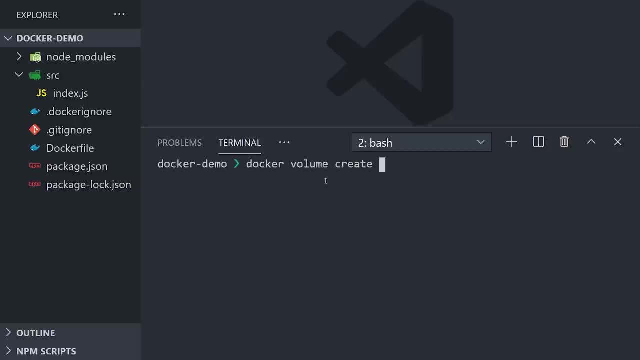 machine And inside this folder, a container can create files that can be remounted into future containers or multiple containers at the same time, So let's go ahead and open up the container. To create a volume, we use the Docker volume create command. Now that we have this volume, 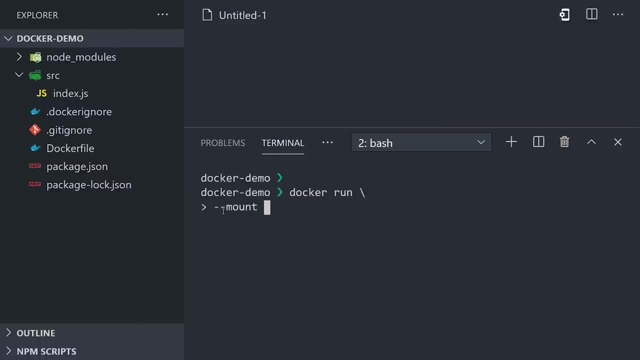 we can mount it somewhere in our container. when we run it, Multiple containers can mount this volume simultaneously and access the same set of files, and the files stick around. after all, the containers are shut down. Now that you know how to run a container, let's talk a little bit. 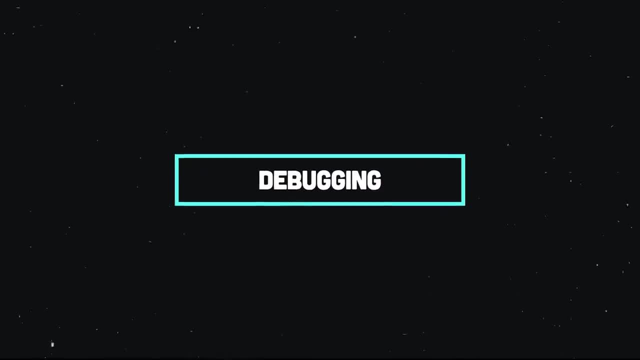 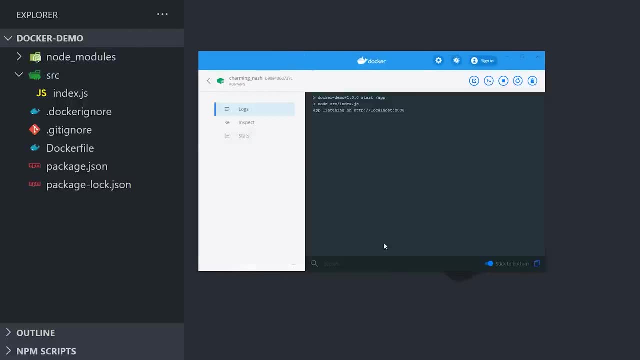 about debugging When things don't go as planned. you might be wondering how do I inspect the logs and how do I get into my container and start interacting with the command line? Well, this is where Docker Desktop really comes in handy. If you click on the running container, you can see. 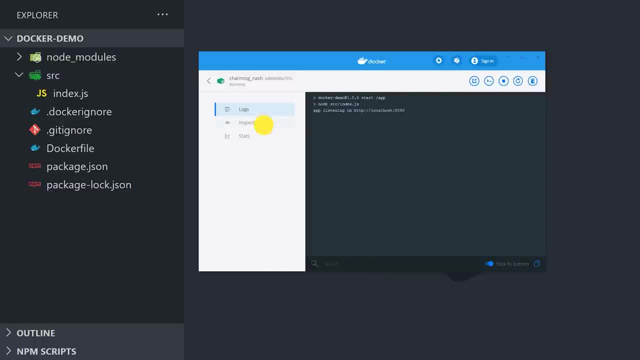 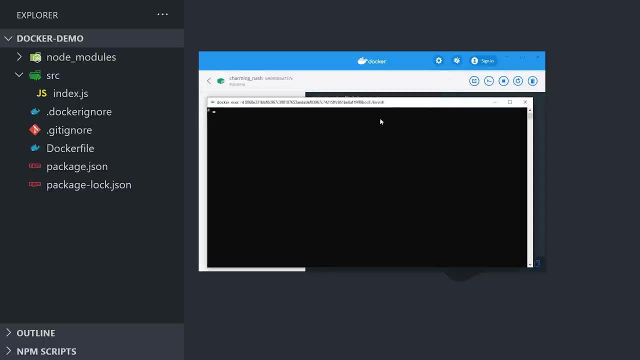 all the logs right there and you can even search through them. You can also execute commands in your container by clicking on the CLI button And, keep in mind, you can also do this from your own command line using the docker exec command. In any case, it puts us in the root of the file system of 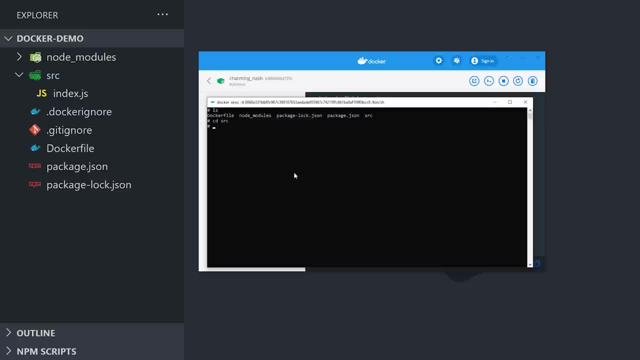 that container so we can then ls to see files or do whatever we want in our Linux environment. That's useful to know, but one of the best things you can do to keep your containers healthy is to write simple, maintainable microservices. Each container should only run one process, And if your app needs multiple processes, 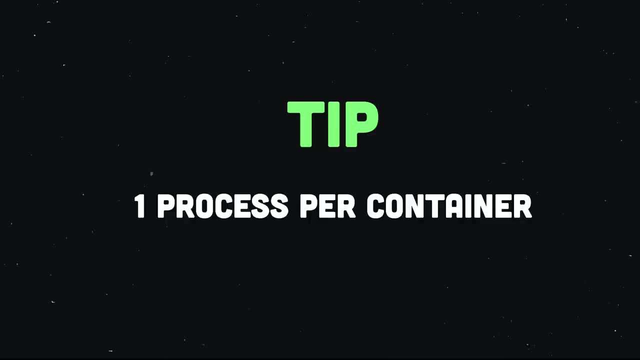 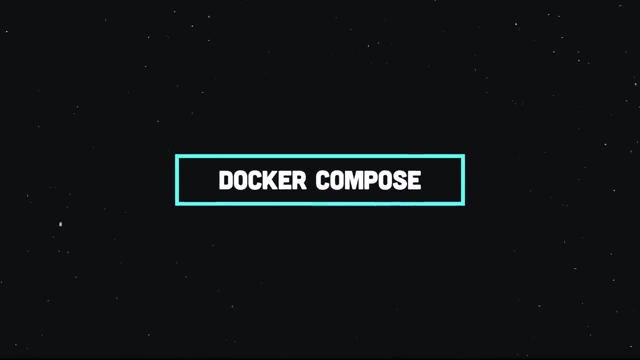 then you should use multiple containers, And Docker has a tool designed just for that, called Docker Compose. It's just a tool for running multiple Docker containers at the same time. We already have a Docker file for our Node app, but let's imagine that our Node app also needs